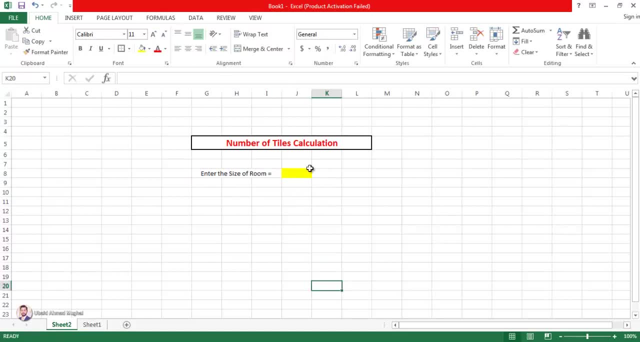 and here you know that we are. we take input in the yellow cells. So here I am going to ask for the length and the units. I am going to write here: fit. I am going to merge this length by width, which is also in fit. I am going to merge this as well. I am going to 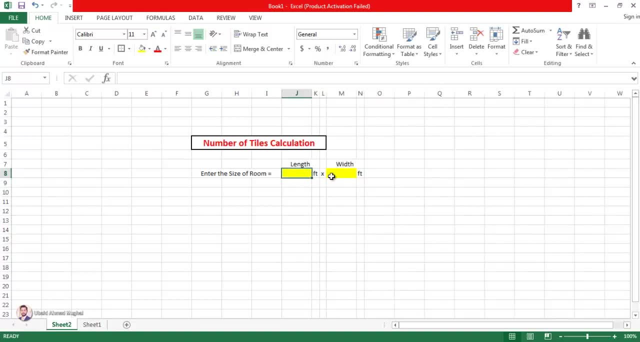 write here fit. So here, whatever the user is going to enter in fit, we have to convert that in inches. So I am going to write this: multiply with 12 to get the answer in inches, and I am also going to do the same thing for this one: This multiplied by 12 to get the 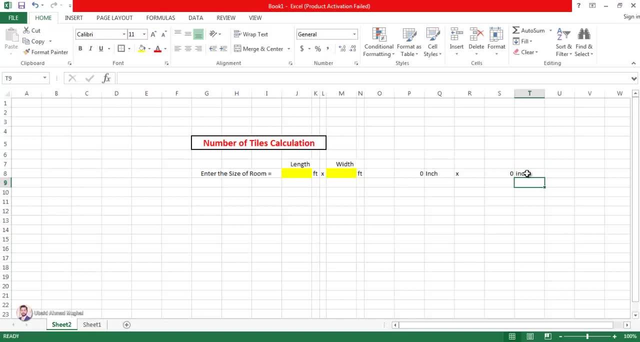 answer in inches. That we are doing because the size of tile we are going to take the input in inches, So that is why we need to convert. So let's see, we enter 10 feet by 12 feet, for example, and the answer is converted into inches automatically. So this is good. So let us- I am going to select. 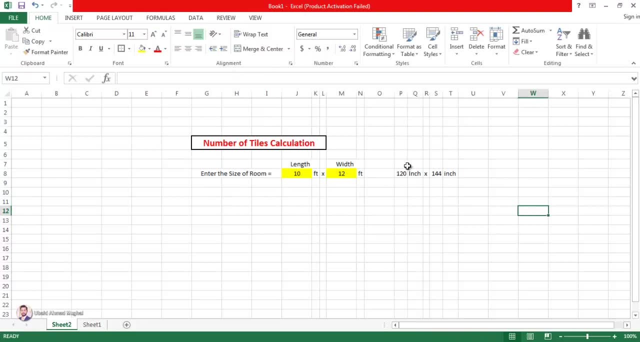 control a and I am going to center align them. Okay, now I am going to enter the size of tile. There are different sizes of tiles available in the market. Two feet by two feet is also available, And 31.5 by 31.5 is also available. Smaller sizes are also available, Whatever size is. 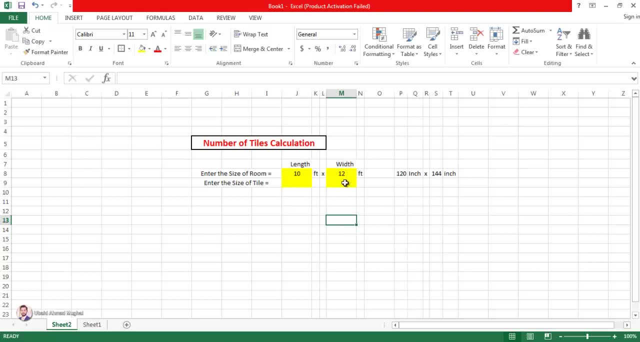 available. you can just enter the size here in inches and it is going to calculate the number of tiles for you. I am going to take the input of the size of tiles in inches, So I am going to write here: inch. double click here to set the width of the column equal. 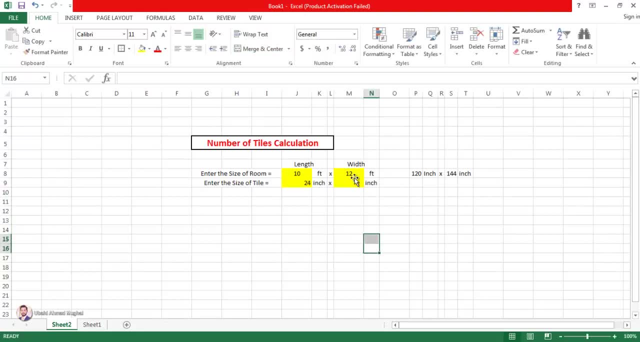 to the text width. So let us say 24 inches by 24 inches is the size of tile which we are going to use. and let's say we don't need to convert here. Yes, we need to calculate the area for the area I am going to write here. area of room is equal. 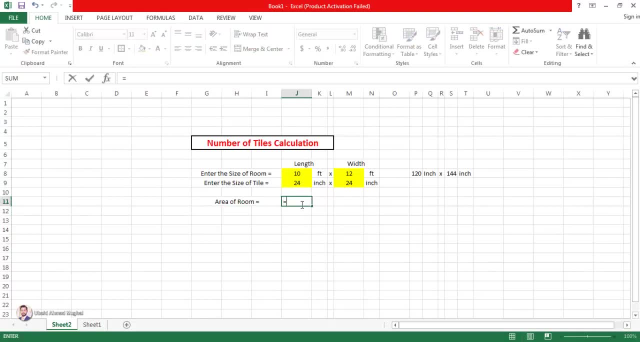 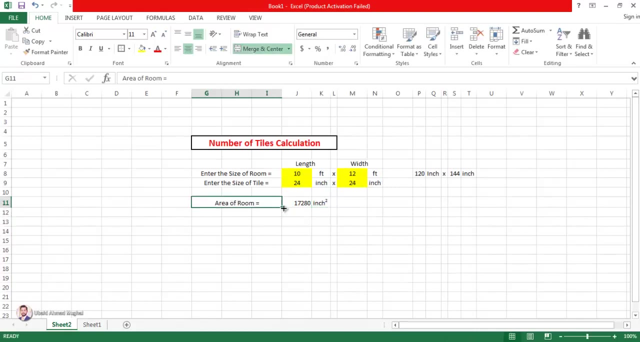 to. so I am going to calculate the area of room in inches, this multiplied by this, and the answer will be in inch square. and I have to convert that to: Okay, Superscript. Okay, Now I have to calculate the area of tile, Area of one tile, And this: 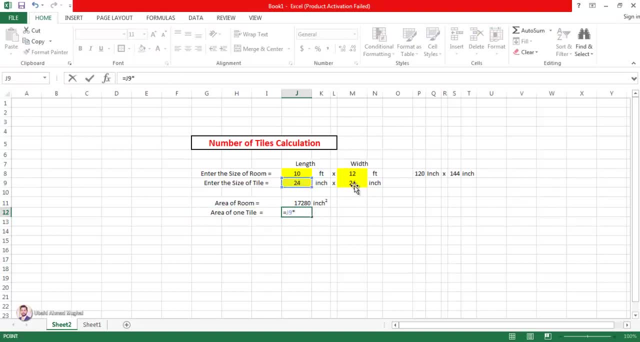 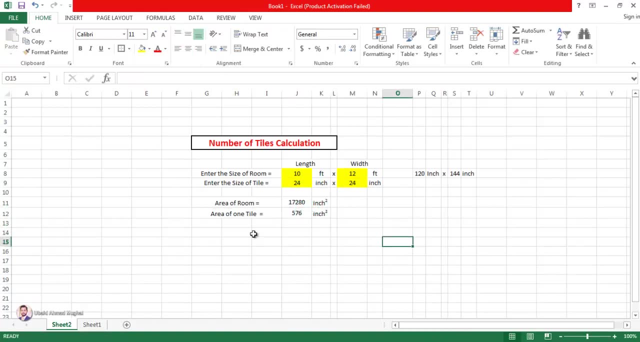 is equal to this, multiplied by this, So you get to know the basic idea that we have to divide the area of room with the area of one tile. It is actually going to give us the person, the number of tiles Which we are going to require to fill that area. Now one more thing is when you are going 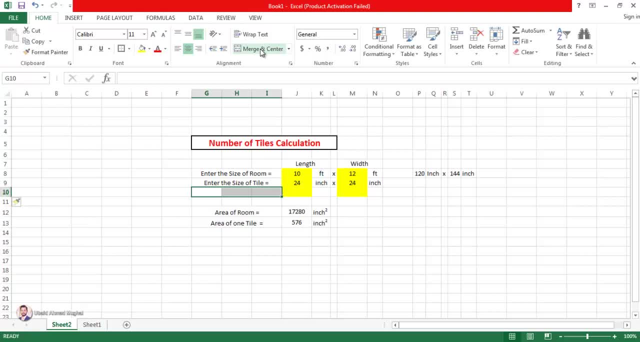 to cut the tiles. If you want to see how to cut the tiles, I have uploaded two videos in which you can see the tile cutting methods and the proper tile installation and the layout procedure. You can go through that videos. I am also going to share the link so you can. 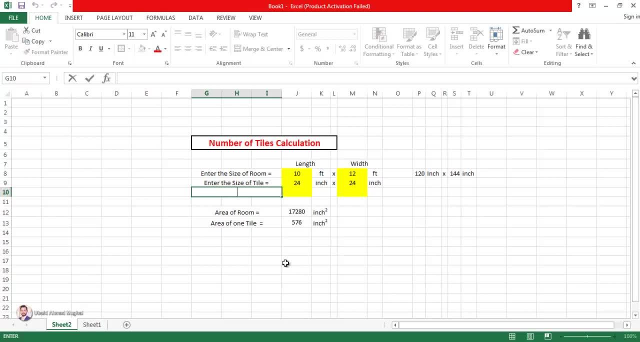 see that the persons are going to waste the tiles, Sometimes intentionally and sometimes unintentionally. the tiles break By some extra tiles and we are going to consider that margin, which is a factor of safety. So I'm going to enter here percentage of wastage. Now it is totally up to you. whatever percentage, 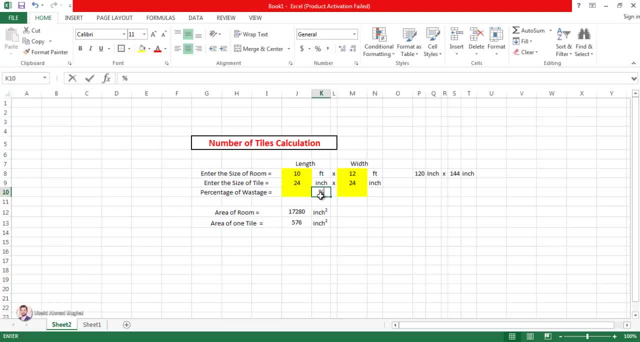 you have to enter here It is going to calculate for you. Let's say, we enter 10 percent as the percentage of wastage, So the number of tiles I'm going to calculate by adding this 10 percent As well. So the number of tiles I'm going to calculate by adding this 10 percent as well. 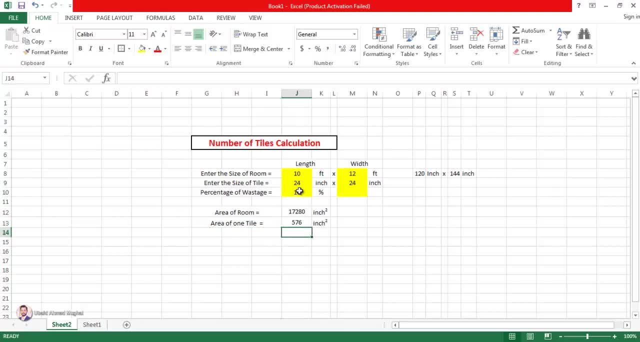 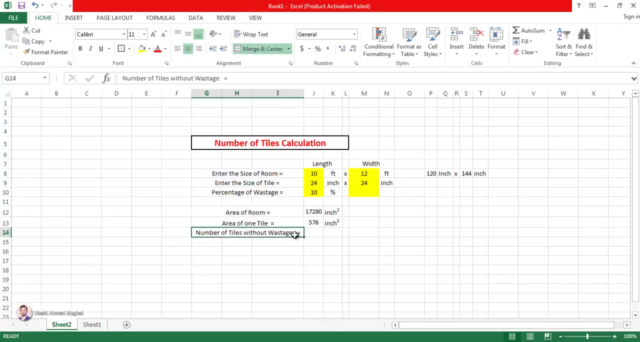 So let us first calculate the number of tiles without adding 10 percent and then let's see, after adding the wastage, how much tiles we get. Number of tiles without wastage. So let's first see this How it is going to be done. 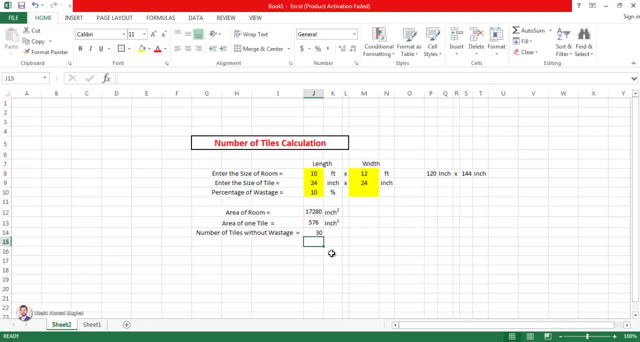 You have to just divide that with Area of one tile. You get 30 tiles. This is your answer without wastage. But it is always preferable that you consider some wastage, because they always break the tiles. So it is better for you to add the percentage of Now this divided by 100. You get to know the 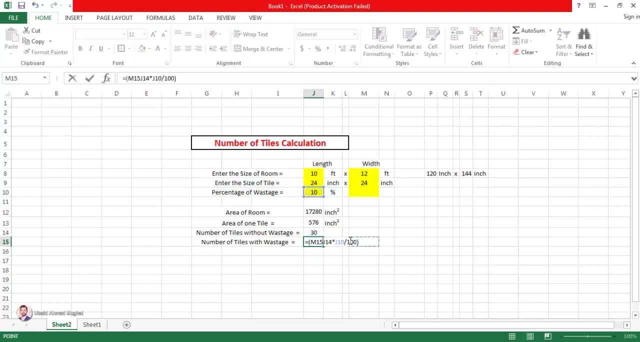 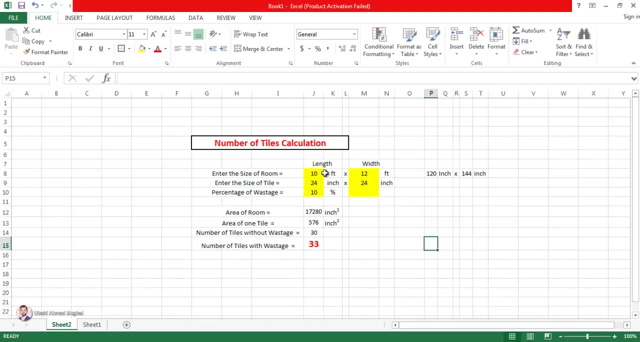 percentage of tiles which are going to be wasted. This I'm going to add with this. So now is the amount of tiles which you have to purchase from the market, which is 33 tiles. It means that a size of 10 feet by 10 feet is going to be requiring 33 tiles off. 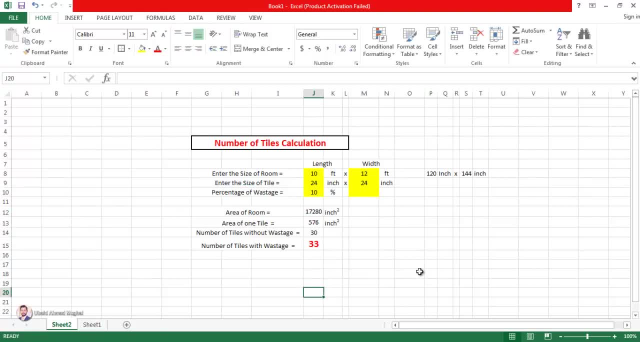 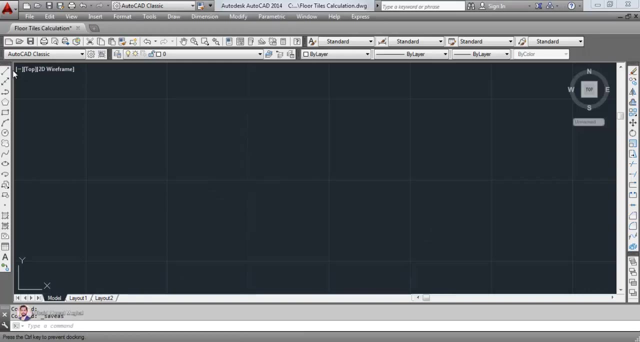 2 feet by 2 feet to be completely placed in that room, to be completely filled. And if you want to verify that, let's just read it further. Okay, we ever do more than to But and fruit and the size of tile is 24 by 24. let's open AutoCAD and try to verify that. I'm going to write here 10. 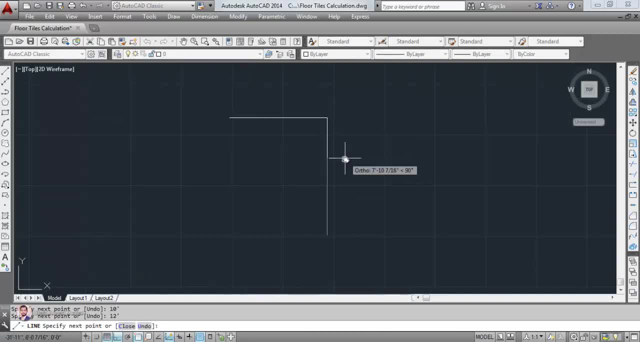 feet by 12 feet. now this 10 by 12, this is going to be my room size. so this is my room and now I'm going to draw a tile. 2 feet by 2 feet is going to be my tile and I'm going 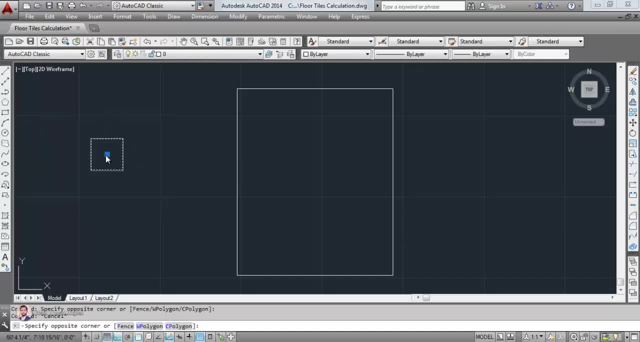 to group this lines into one huh box or one object which I can easily place. so I am going to move that from this corner to this corner. now I am going to copy that. I'm going to see how many tiles are actually required to fill this room and whether our calculation is correct. 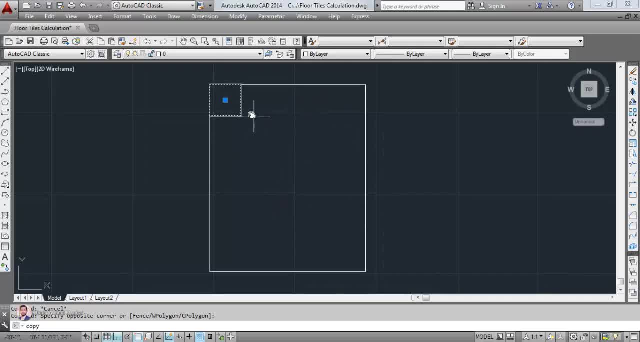 or not. So, while copying them, I'm not going to use these spaces, the tiles, because, because these are very small, and this is usually 2 millimeters to 3 millimeters, it is very less and you are actually going to require a tile a. 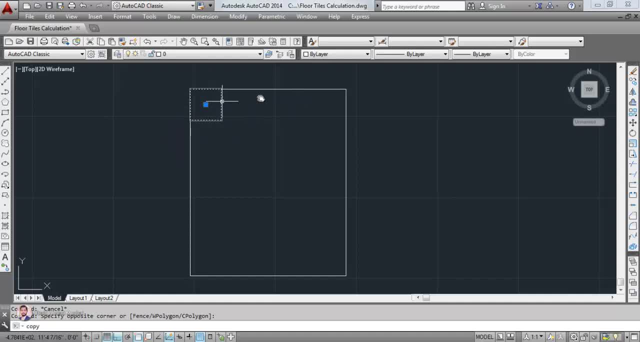 bigger tile because, when you are going to consider, the spaces are- well, it is- it is not going to be enough, so that it is going to save you one tile, complete. no, it is not going to happen, so you have to purchase the complete tile. that's why it. 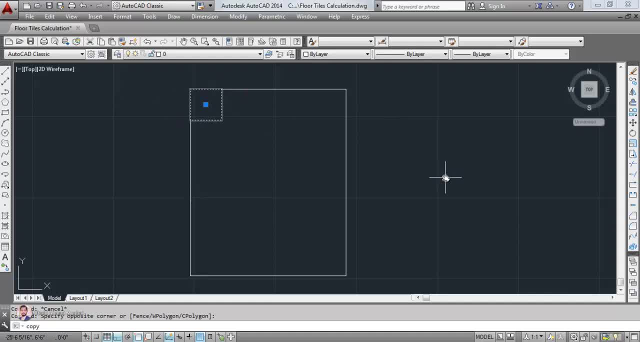 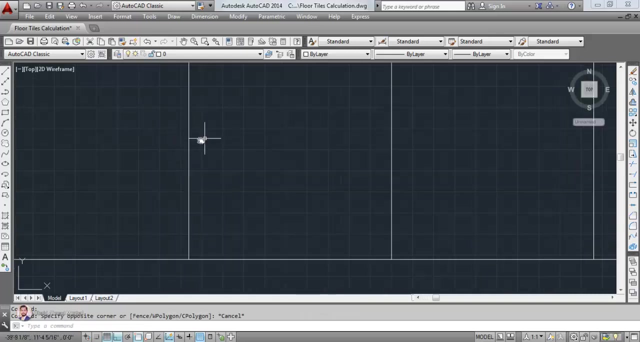 is going to be on our benefit that you purchase more tiles which are actually going to be used in your placement. so I'm going to copy this and I'm going to select M as a multiple copying objects. so just going to click and these are actually 100% correct. so if you just just going to place a 2 millimeter gap, 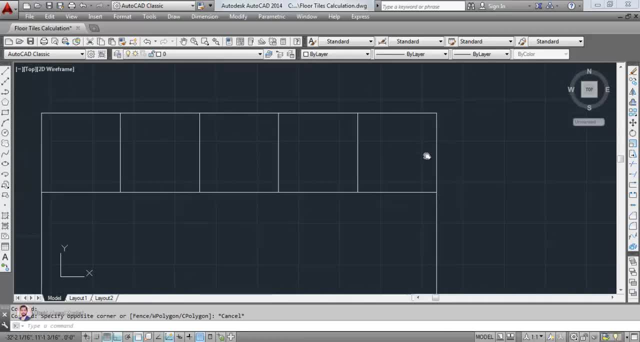 here as well. so this tile is going to be moved to the right side- 2 plus 2 plus 2 plus 2, so 8 millimeters. it is going to be placed to the right and it is going to be cut to the right and it is going to be cut. 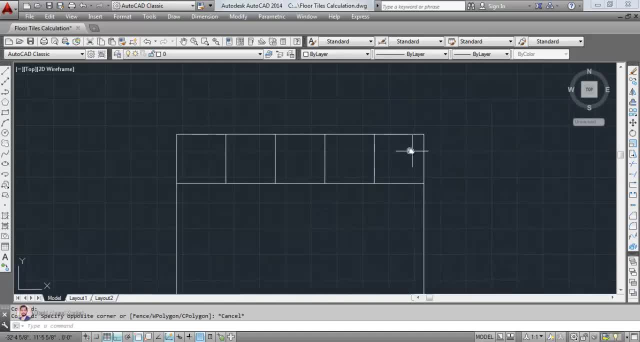 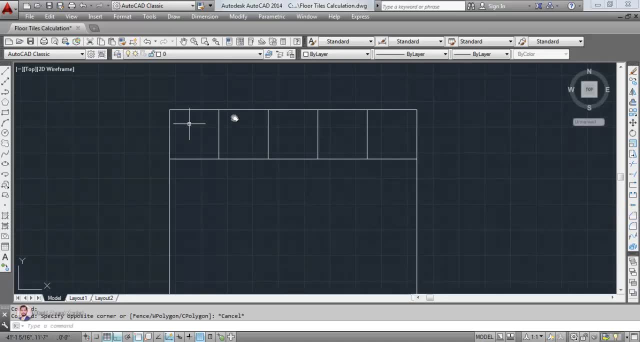 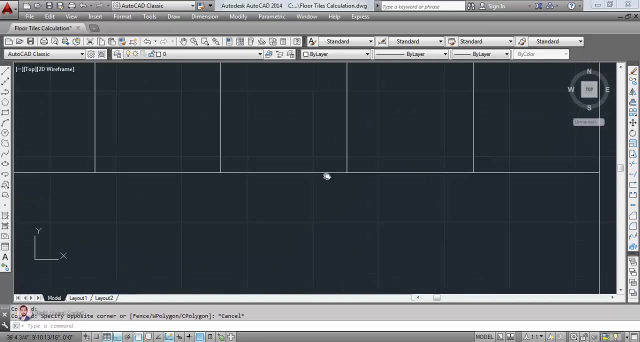 so you are. you are not required to do this. you can either manage the margin by both tiles or you can just place them according to your own requirements. both tiles should be, you can say, placed. sometimes the persons who are going to place their tiles, they don't actually leave the margin, but I don't prefer that. 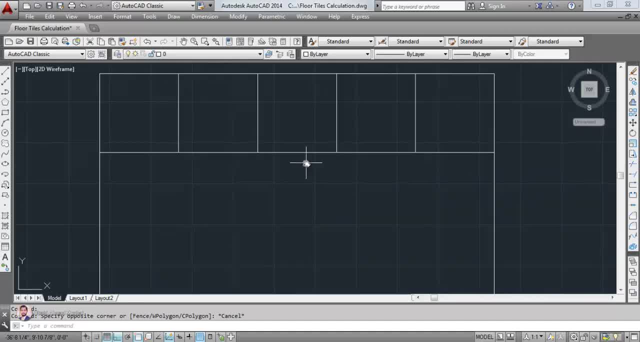 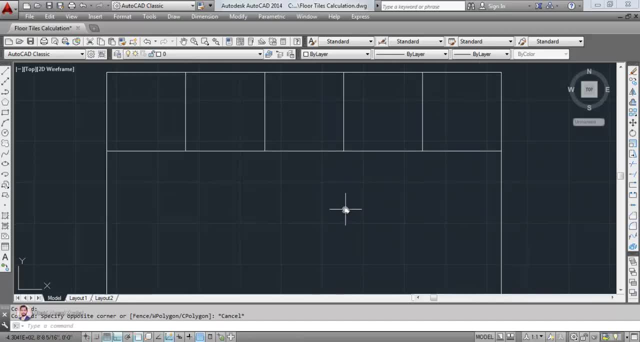 because the problem is the tiles pop up and I have uploaded a complete video on that- how the tiles pop up and how do you feel about that and how to repair that. you can also see the video in my YouTube tutorials. you can see them and can see why the spaces are required or the spaces are. 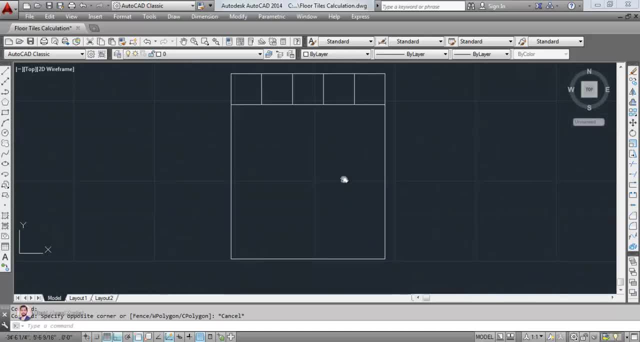 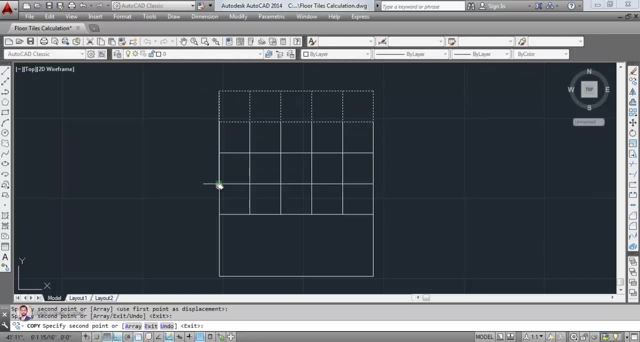 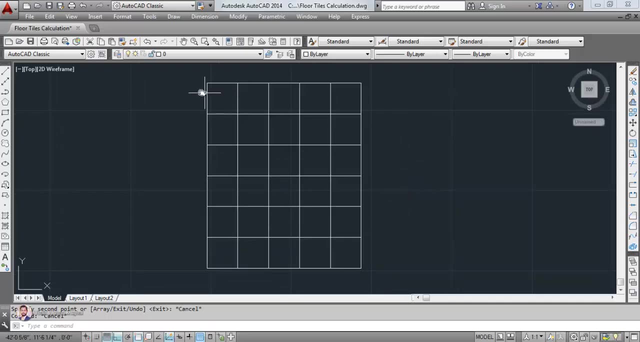 required in between the tiles. so these are one, two, three, four, five, five tiles and we are going to see how many tiles are actually required to complete this 10 feet by 12 feet room. I'm not going to copy them and these are 100% filling the area. so one, two, three. 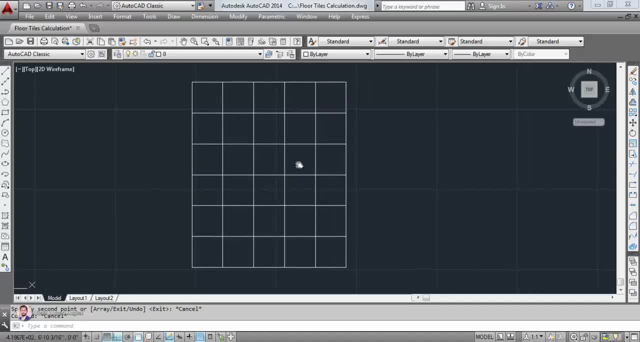 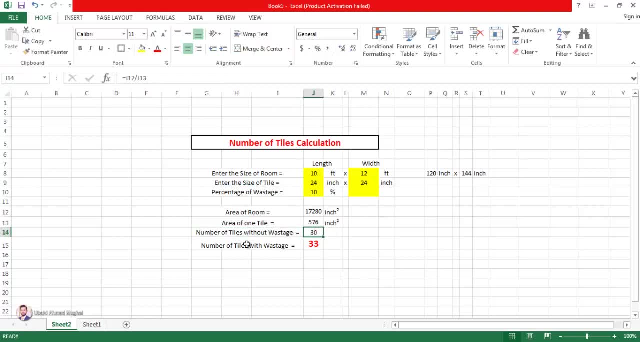 four, five and one, two, three, four, five and one. two, three, four, five and one, two, three, four, five, six, five, six thirty. so we have 30 tiles here. so in our calculation, 30 tiles without any wastage. so if you see that you just require 30 tiles to be, placed and if there are some doors, some irregular shapes there, those require cutting and when they cut they can damage the tile. sometimes, while handling the tiles they can cut. if work is performed 100%, 100% correctly, then you don't require any extra tiles. so it is always preferred that you buy some three to four. 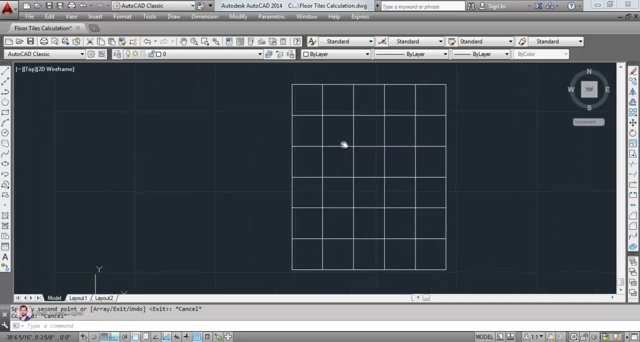 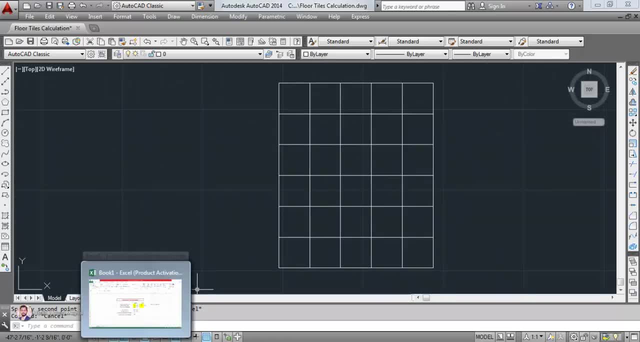 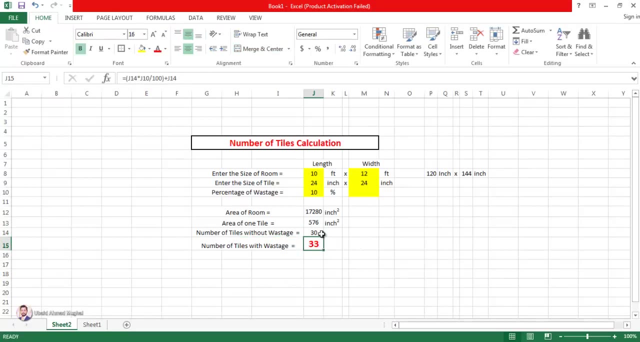 tiles, extra tiles or, depending upon the you can say- the shape of the complexity of the room, the amount of cutting required. it is going to tell you how much tiles you require. so here, the number of tiles with wastage are shown to you as 33. so this is a very simple. 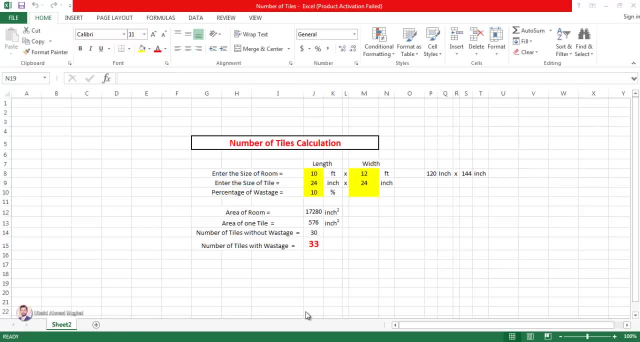 procedure: how to calculate the number of tiles. okay, now we have the number of tiles required, so we want to calculate the cost of the tiles required as well. let us continue with the cost of the tiles required. so cost of tiles is going to be see. first of all, I'm going 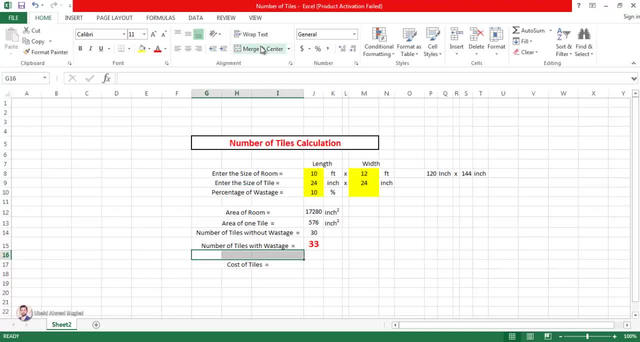 to enter the cost of one pack of tiles. packet of tiles. cost of one packet of tiles is going to be equal to. so it depends which brand you are taking and what. what is the design of the tile and what is the quality of the tile. so from the market you can get. 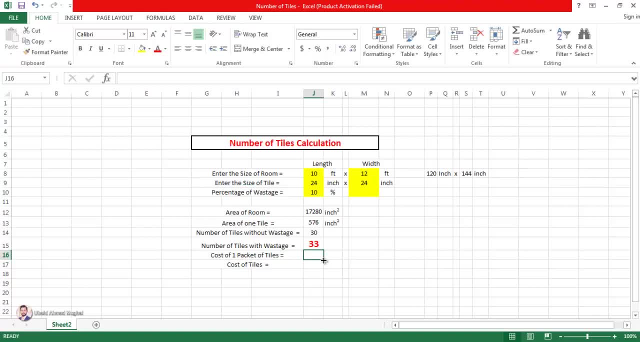 the idea how much is the cost of one packet of the tile. one packet of the tile is equal to one point four, four meters, so one point four, four meters, and it contains four tiles of two feet by two feet. I can show you the picture as well. 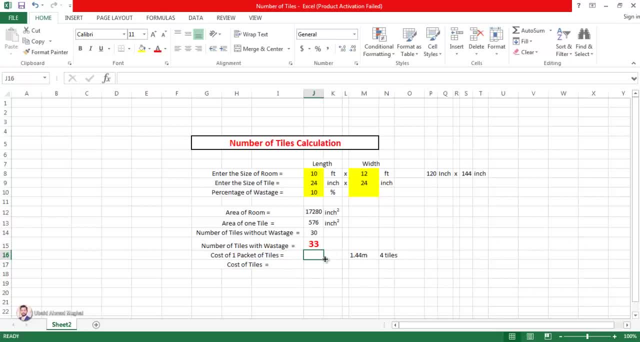 if you want to enter the rate, input rate here. so let's say it is around three thousand rupees Pakistani, the one which I bought, the cost of tiles. this is equal to you require how many boxes now, because one packet contains four tiles, and the amount of tiles which you 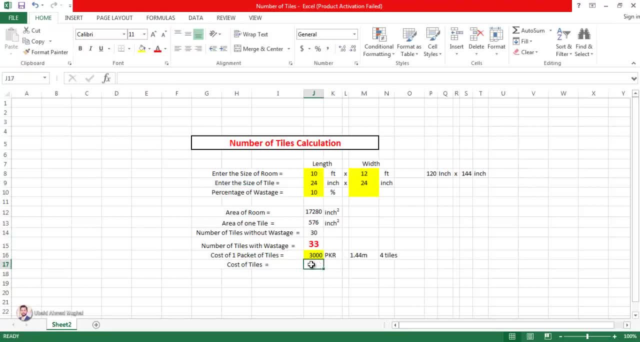 require is 33.. so this is equal to divided by four. you get eight point two five. so you have to round it off to the upper side so you can write it round up here you have to write the number of digits of zero. so nine packets you require with the, you can say, factor of safety, if you 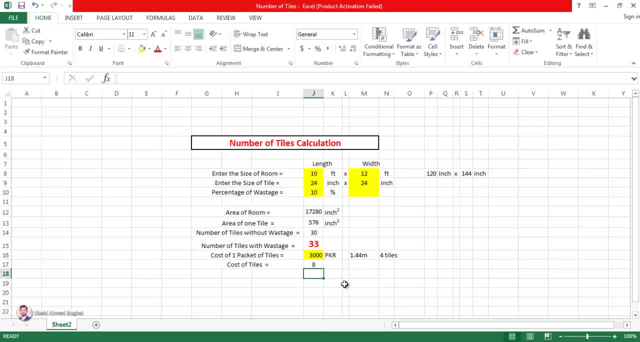 don't consider the factor of safety and then you want to see: then only eight packets you require, but it is always preferred that you keep the cap. a factor of safety here. the cost of tiles, number of packets are this one I am going to write: number of packets required are nine and the cost of tiles will be nine.